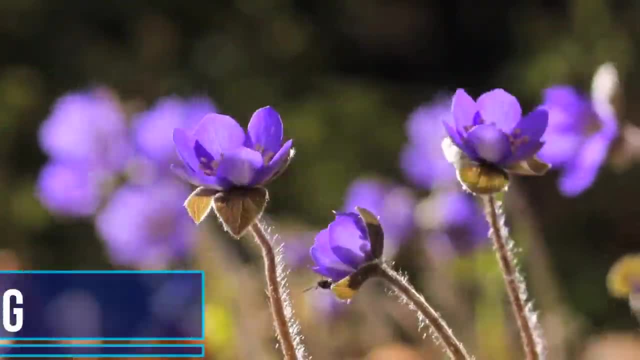 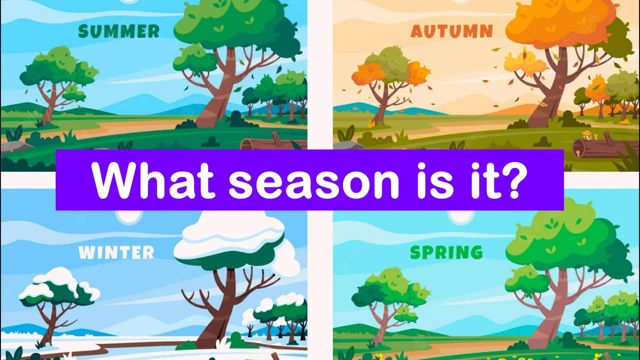 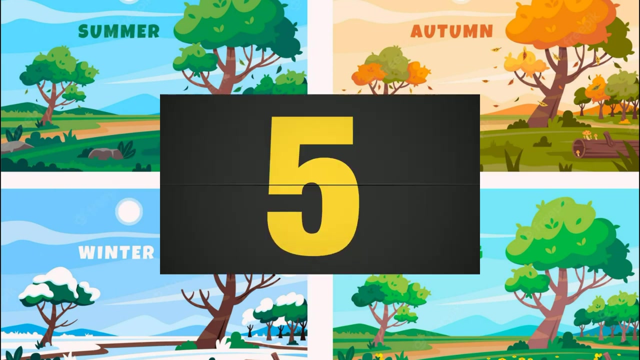 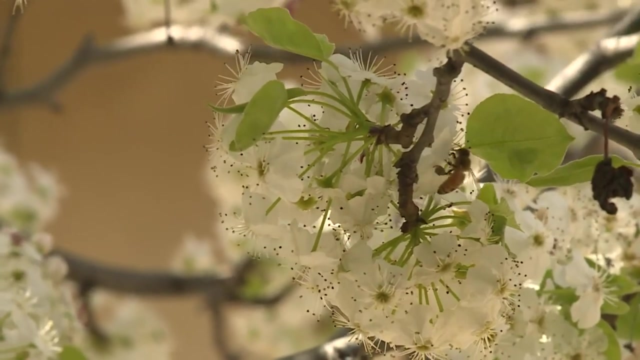 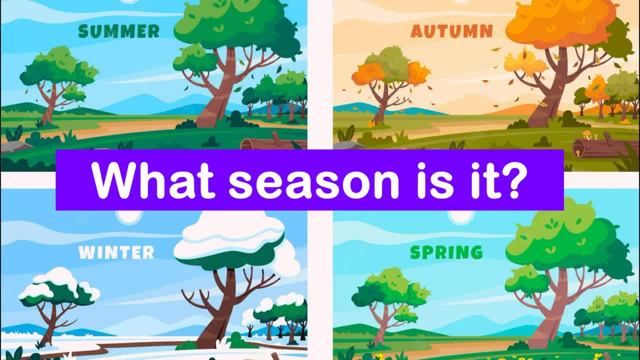 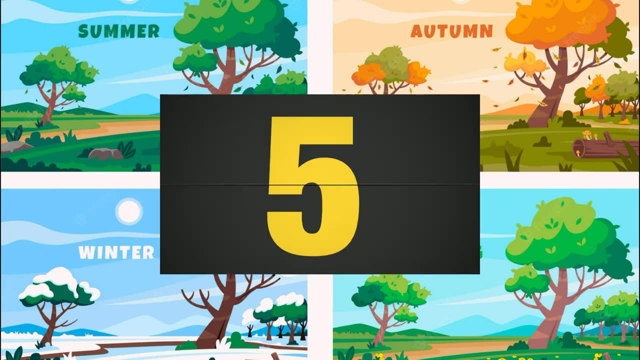 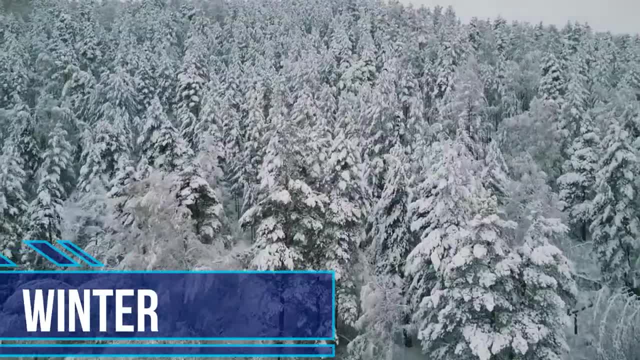 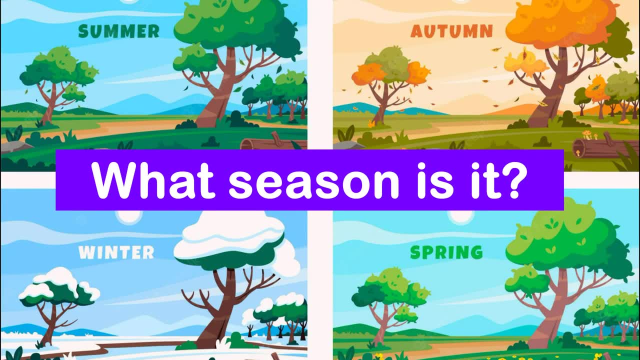 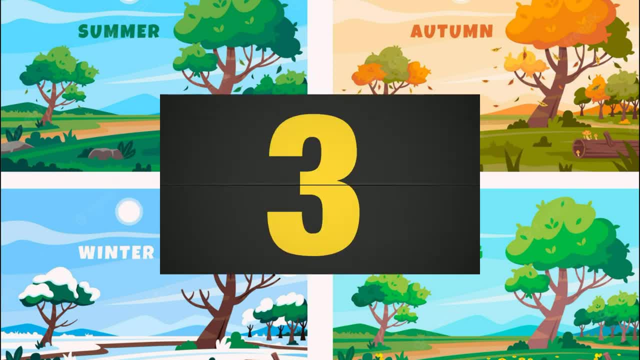 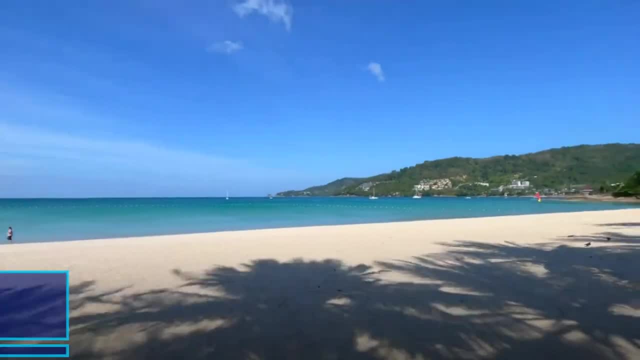 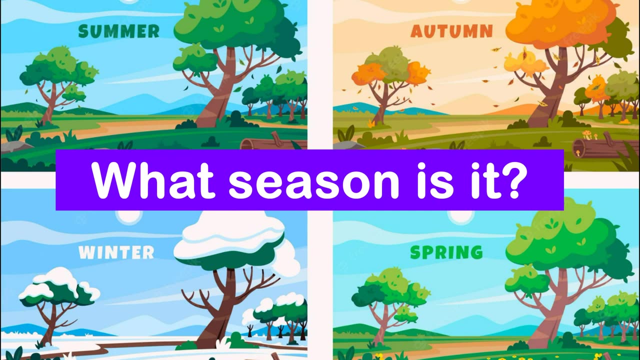 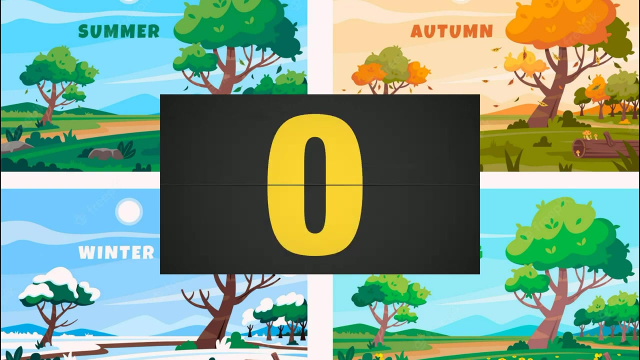 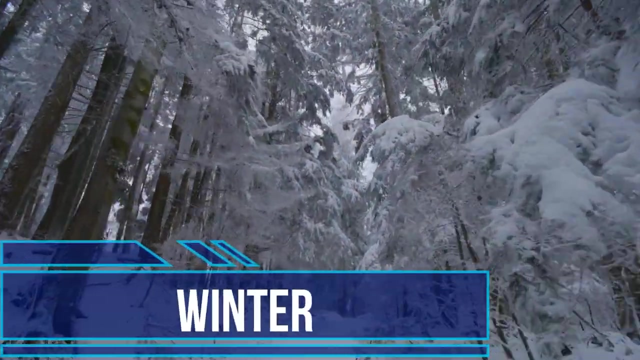 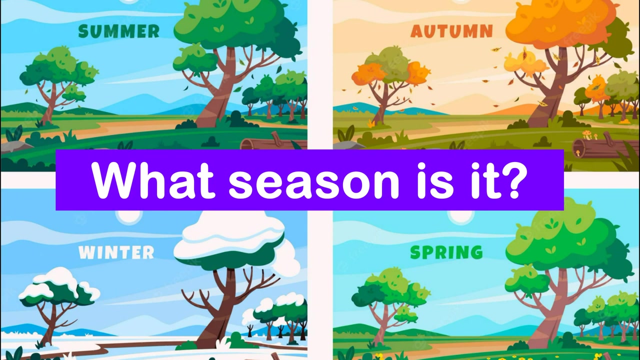 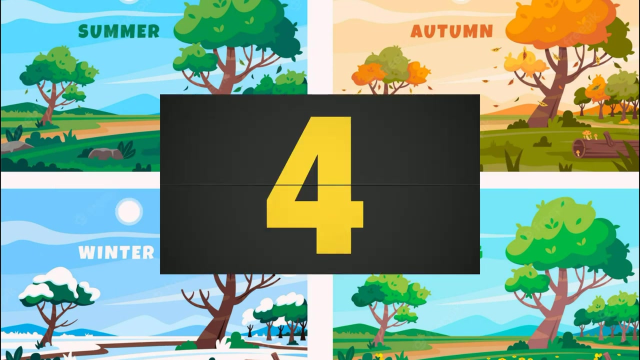 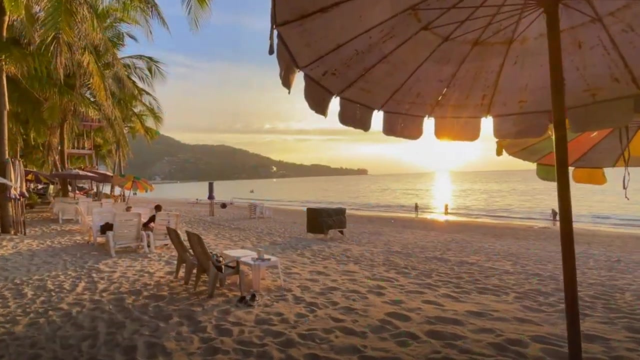 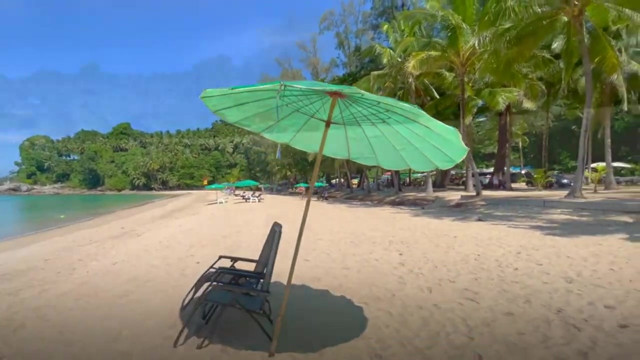 When there's snow on the ground, you can make a snowman There. It's warm every day. The nights are warm too. Sometimes it's very hot. When it's hot, it's fun to go to the beach. It's fun to rake the leaves into piles. 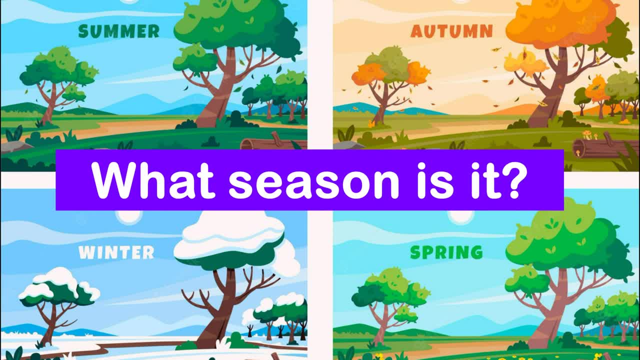 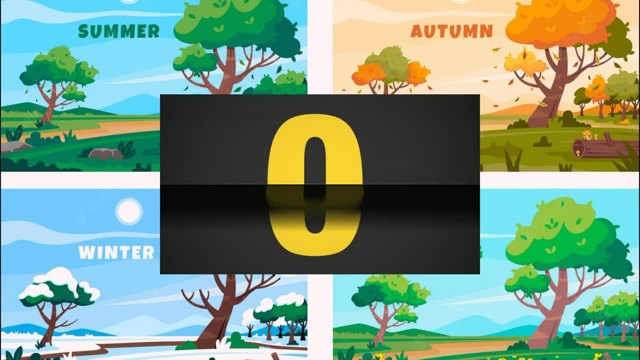 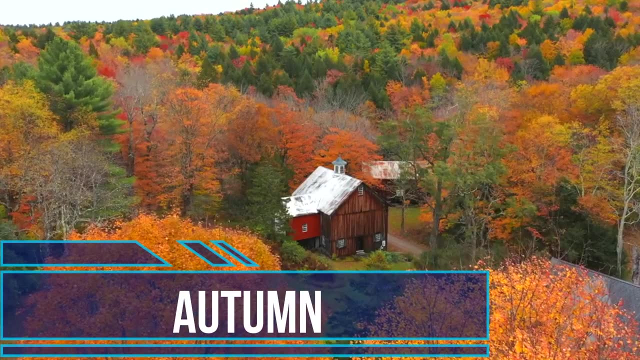 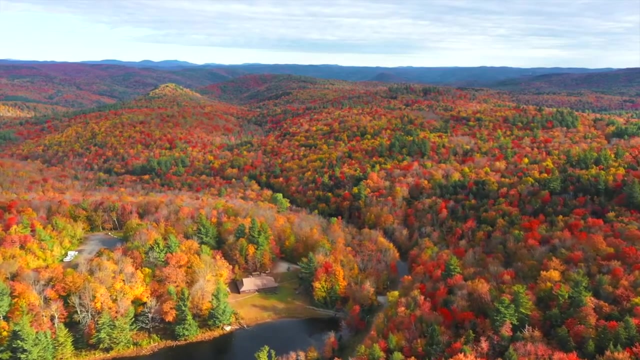 You can jump into a pile of leaves. It's fun to rake the leaves into piles.